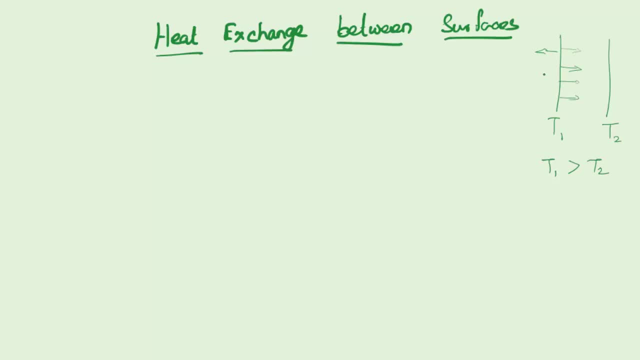 radiation from this in all directions. So the radiation in this direction will be absorbed by this plate because of the temperature of this plate is lesser than this plate. ok, So in case, consider, T2 is greater than T1, then the radiation emits by this surface will be absorbed by the 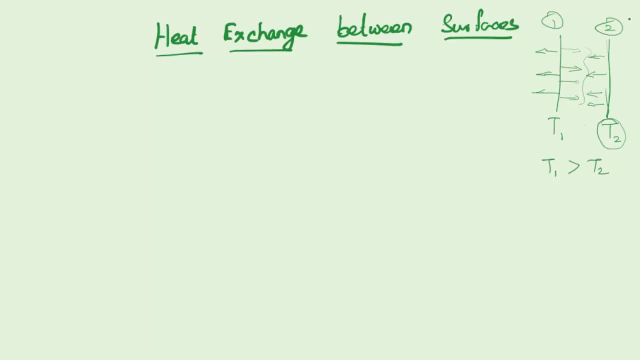 first surface, number 1, this is number 2 surface like this. So now consider: So: first formula is heat exchange between two large parallel plate, heat exchange between two large parallel plates. ok, So now Q 1, 2, since I am considering surface number, 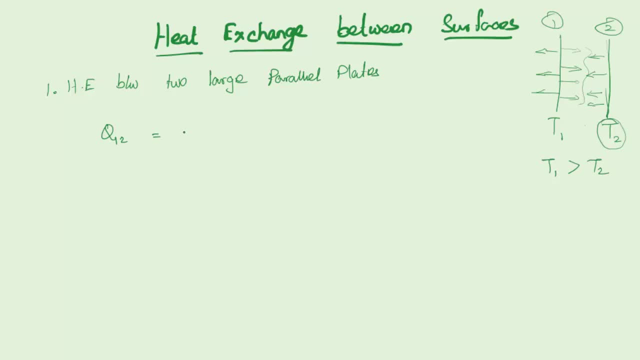 1 and the surface number 2, this is Q 1, 2 equal to epsilon, to the power bar T2.. So sigma A into T1 to the power 4, minus T2 to the power 4, ok, Now where epsilon bar. 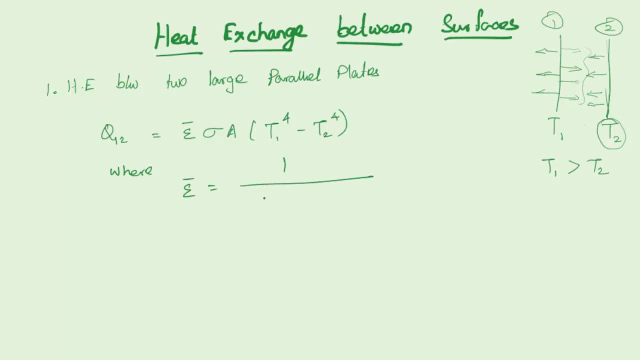 epsilon dash equal to 1 divided by 1. divided by epsilon 1 plus 1, by epsilon 2 to the bracket minus 1, this is the formula for epsilon dash. Similarly, the second formula is heat exchange between two large concentric cells. So this is the formula for heat exchange between two large concentric cells. 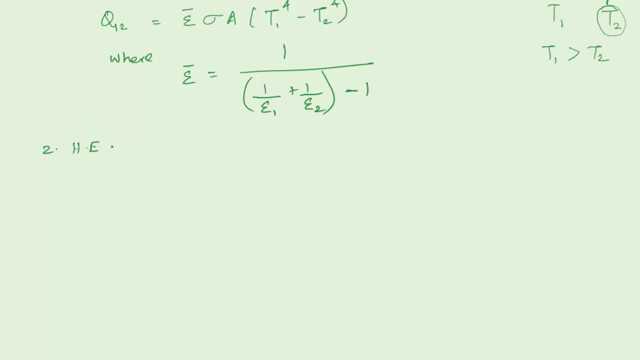 So it is heat exchange of cylinder or spheres. heat exchange between cylinders are spheres. ok, Now the formula is: Q 1, 2 is equal to epsilon, bar A1 sigma into T1 to the power 4 minus T2 power 4.. Now here epsilon value is equal to 1 divided by 1 divided by epsilon. plus A1, comma, delta T2 to the power 4 plus one plus a, 1 plus x minus x. So you look here for this 해주. this is the formula for wij y: equal, equa1, equa2, equa1, equa2, equa2, remember. to put this changes. So the normal value here is this: epsilon value is equal to 1 divided by 1. divided by 1 divided by epsilon plus a1� Yi cube, But effects is generallyacci hoped 0.. Or at sign of in this example you can say: choose again With this highest. 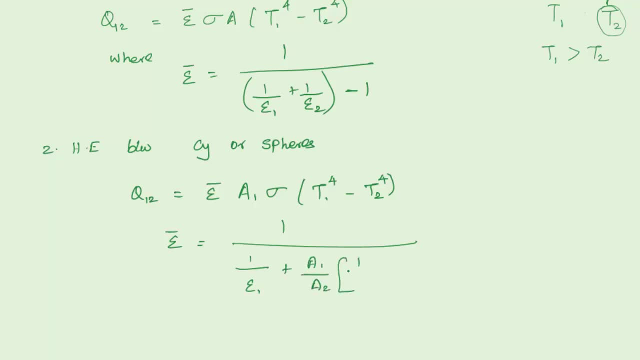 a 1 divided by a 2 into 1 divided by epsilon, 2 minus 1. ok, Here the a 1 value- sorry, the a value is 2 pi r L for cylinder. Similarly a equal to 4 pi r square for sphere. So if 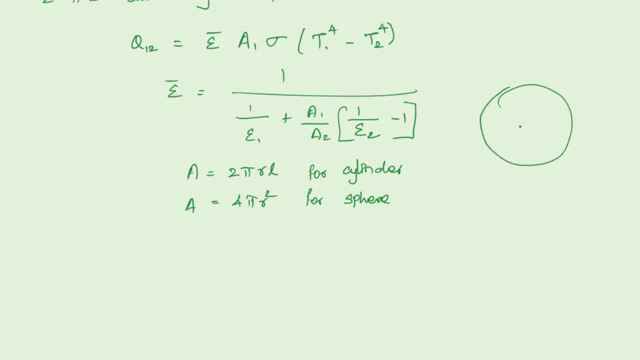 you consider concentric cylinders like this. So the inner area is called as a 1, the outer area is called as a 2.. For both a 1 and a 2, the formula is 2 pi r L. The r value will. 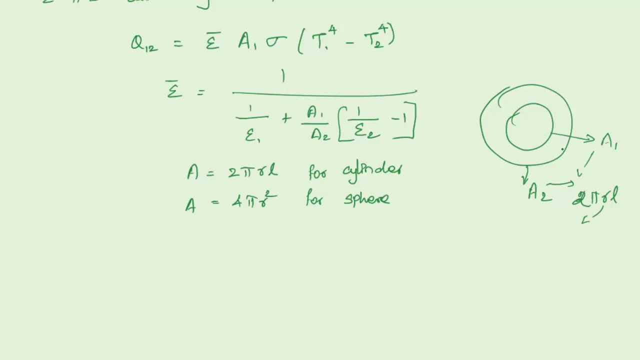 differ for the inner cylinder and outer cylinder. So this is the second formula. The third formula is heat transfer with n number of shields in the is given by heat transfer with n number of shields. n number of shields. ok, this is q 1- n, So number of if you use two numbers of shields. 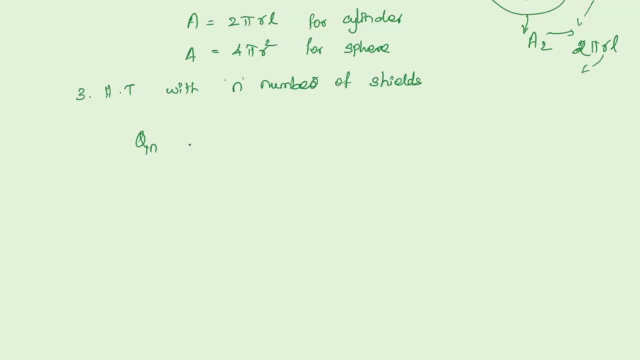 in the sense you have to substitute q, 1, 2.. So here, which is equal to A, into epsilon t 1, power 4 minus t 2 to the power 4 divided by 1, divided by epsilon 1 plus 1 divided by. 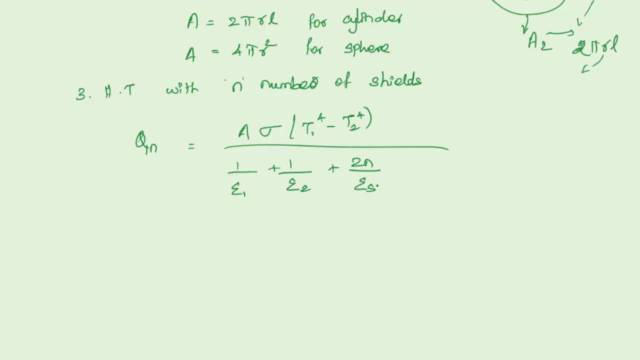 epsilon 2 plus 2 n, divided by epsilon s minus n plus 1. ok, Here, epsilon 1 is the surface emissivity, epsilon 2 is the second surface emissivity and epsilon s is the shield emissivity. So if you have three number of shields, all three number of shields will have three number. 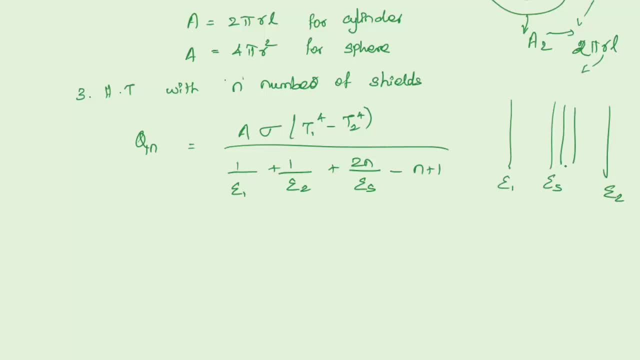 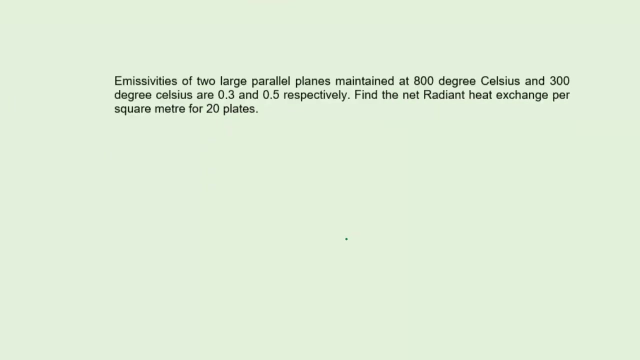 of shields. So you have equal emissivity value. ok, Similarly, n equal to number of shield. ok, with all these formula we will solve the problem. So go to the first problem. So this is the first problem given. So in this problem, emissivity of two large parallel plates maintained at 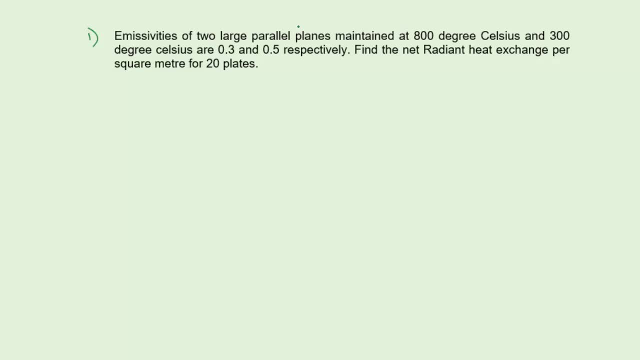